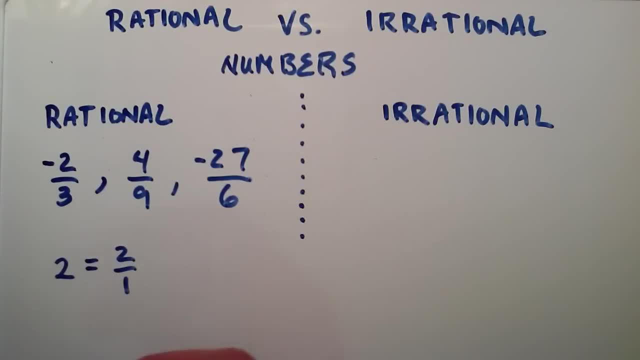 the integer three can be written as three divided by one, and so on. You can divide any integer by the number one and you can write it as a ratio of two integers. So because of this property, all of the integers are also rational numbers. 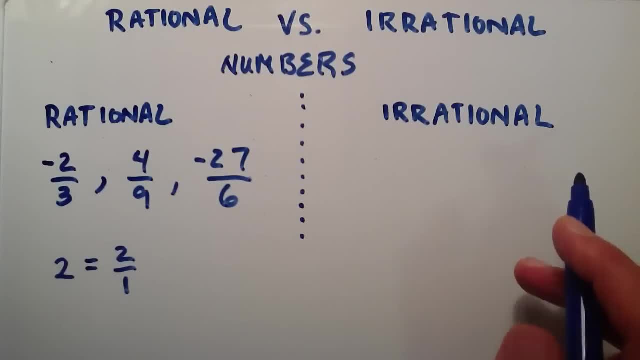 So what is an irrational number? Well, an irrational number is all the numbers in the real number system that cannot be written as a ratio of two integers. So those types of numbers are numbers such as the square root, the square root of two, the square root of five and the square root of seven. 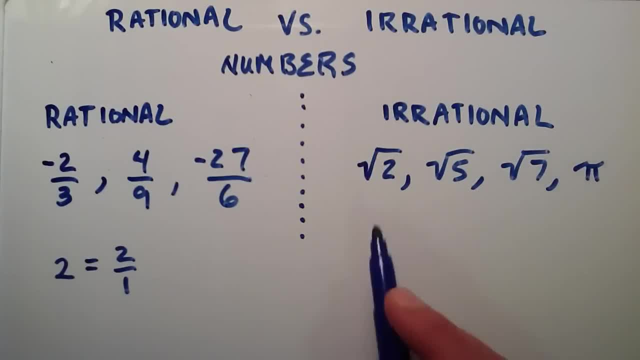 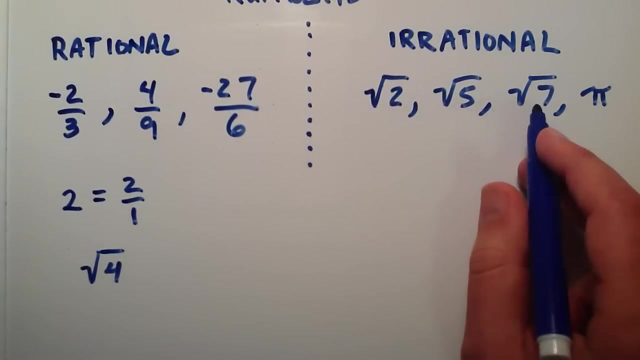 Also, the number pi is an irrational number, So none of these numbers can be written as a ratio of two integers. therefore they are irrational. So what about something like the square root of four? Well, the square root of four kind of looks like the numbers I've written here. 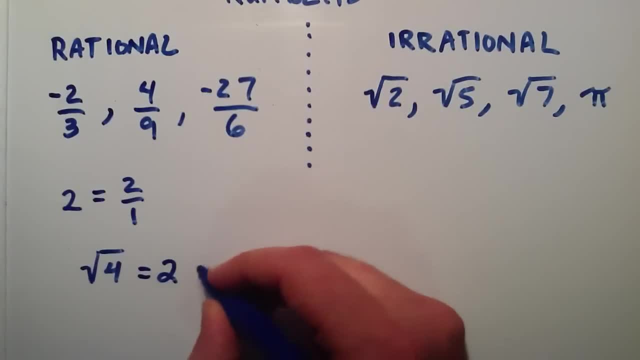 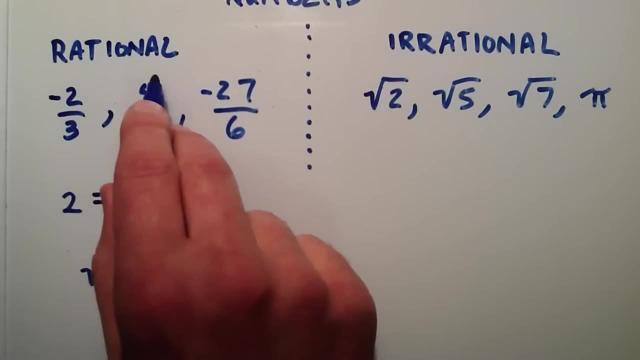 but the difference is the square root of four can be written as the number two and the number two can be written as a ratio of two integers. The square root of four is actually a rational number. So that's the difference between rational and irrational numbers. 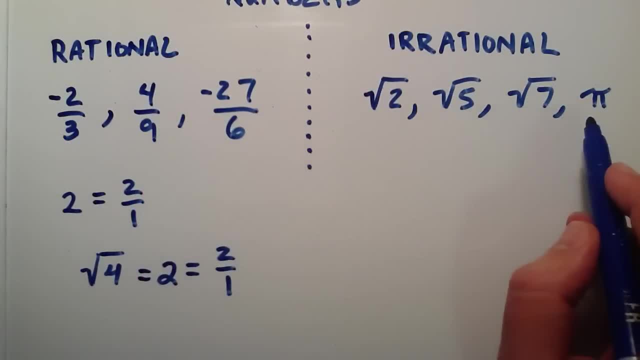 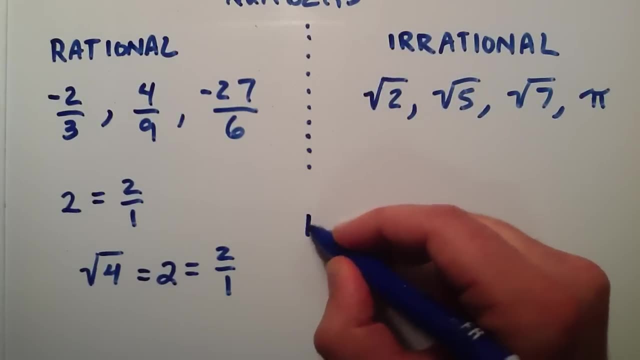 One can be written as a ratio of two integers and the other cannot. And if you take all of the rational numbers and add them to all of the irrational numbers, then you get what we call the real number system, And the real number system is often denoted by this symbol. 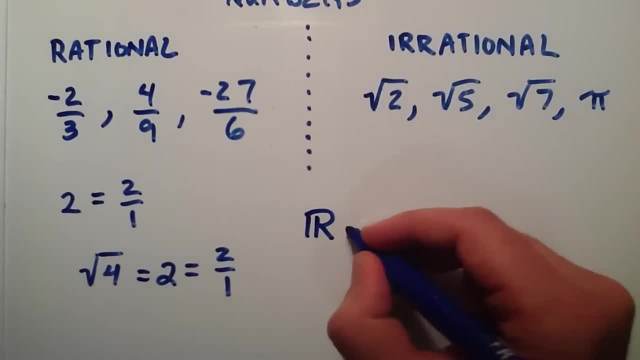 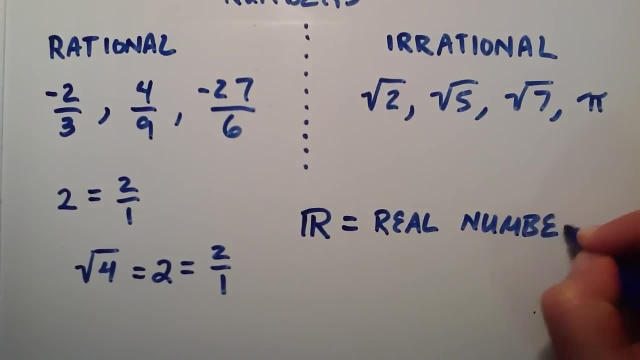 It's like an R with an extra line on the left side, So let me just go ahead and write that. So this is the real numbers And you might see this in your courses that you're taking The real number system. 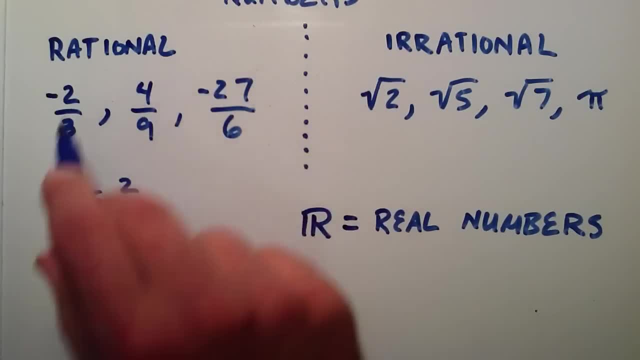 And so yeah, basically, the real number system is all of the rational numbers plus all of the irrational numbers in one big group. So anyway, this video explained the difference between rational and irrational numbers and the combination of all these numbers together. 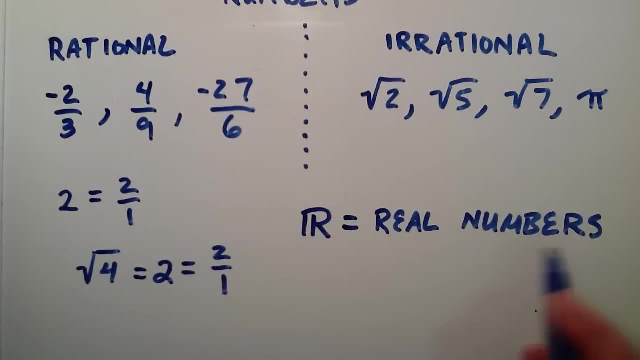 going to one group that we call the real numbers. So thanks for watching. Stay tuned for more tutorials in the intermediate algebra playlist And if you haven't done so already, don't forget to subscribe.